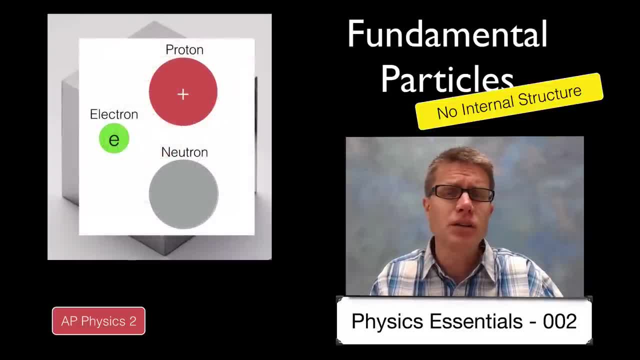 itself is made up of protons and neutrons. And if we look into those protons and neutrons, you may not know it, but they are made up of quarks themselves. A proton is made up of two ups and one down- quark. And a neutron is made up of two downs and one up quark. 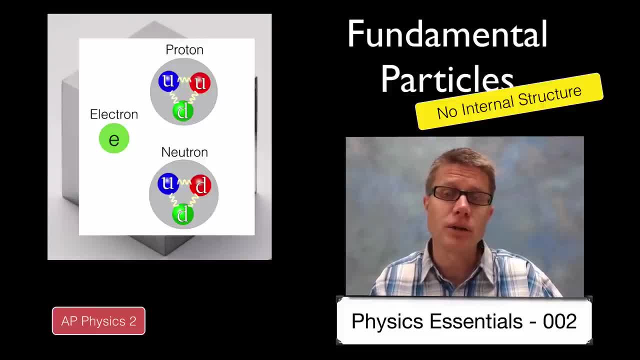 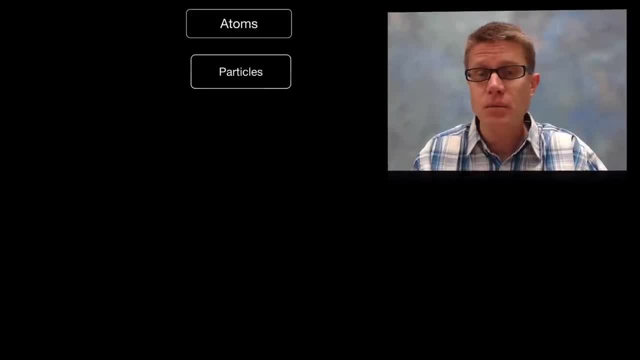 And so when we finally get to the level of quarks and electrons, we are at the level of fundamental particles, In other words particles in physics that have no internal structure, And so atoms are made up of subatomic particles- Electrons, protons and neutrons, And not all of these. 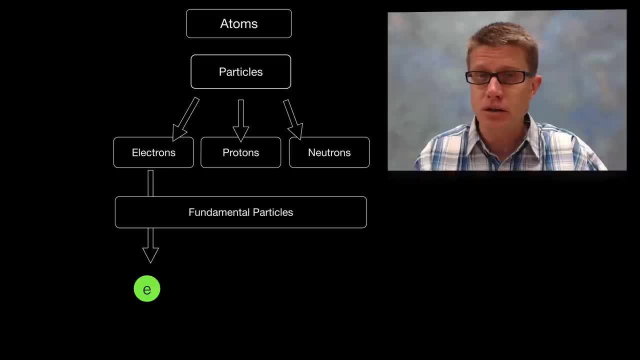 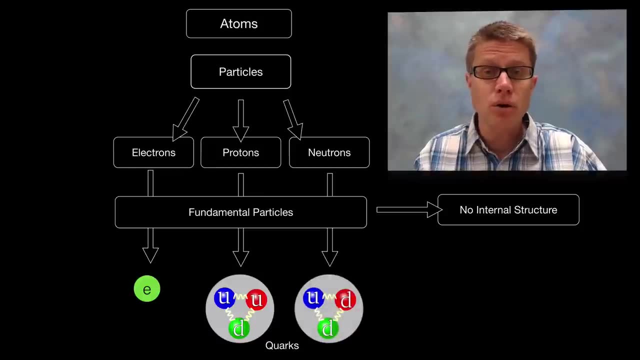 are fundamental particles, And so an electron is because it has no internal structure. But protons and neutrons are made up of quarks, And those quarks themselves have no internal structure, And so they are fundamental, But the protons and neutrons are not. Now, when? 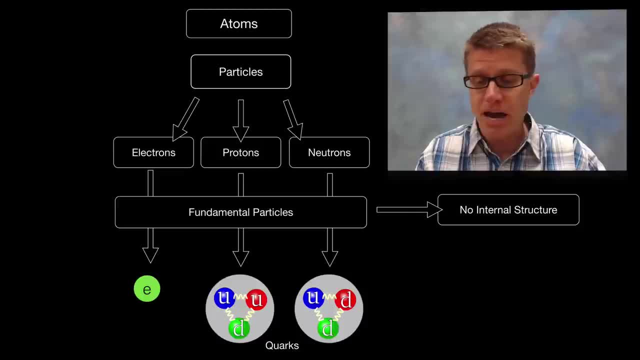 you get to the level of the quarks, we will find that they have properties. They have properties like mass and spin and charge And we can sum up those charges and it tells us a lot about the overall charge of the protons and the neutrons. What are some other fundamental 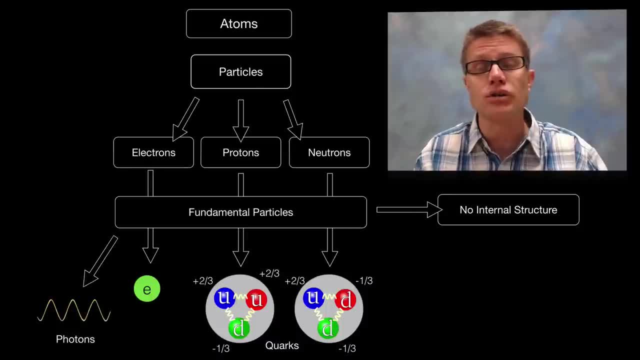 particles. Photons are going to be little quanta of light or electromagnetic radiation. Neutrinos are another type of fundamental particle, And so what makes up matter at the smallest level are these fundamental particles, And so you can think of that cube of purified 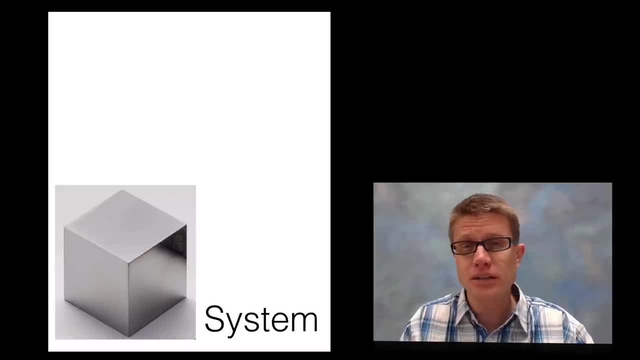 iron as a system made up of electrons, neutrons and neutrons, And if you think about this, So that's the temperature that we have, If you think about the temperature of, really, of other objects, And we have to dig into that system to find the most fundamental of. 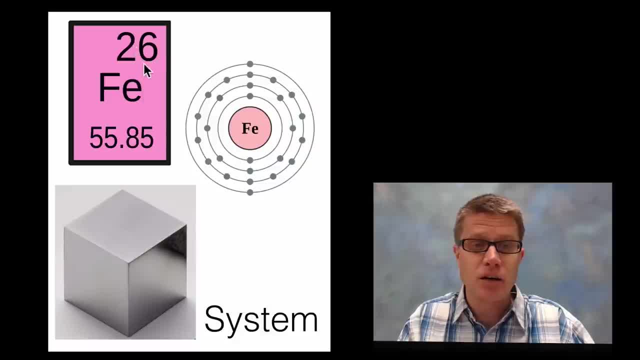 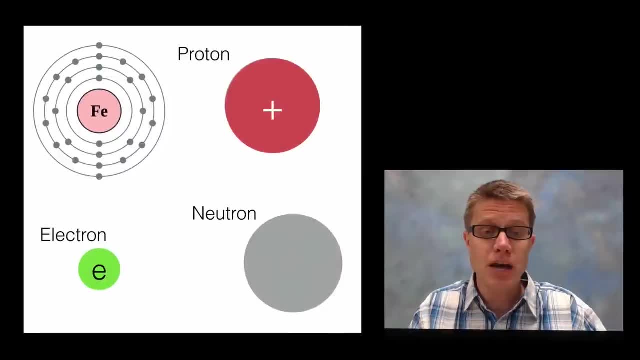 those objects. We know that in a sample of iron there are going to be 26 protons And then we are going to have about 30 neutrons in a typical nucleus. As we zoom into that we finally get our first fundamental particle, the electron. But we have to dig farther into. 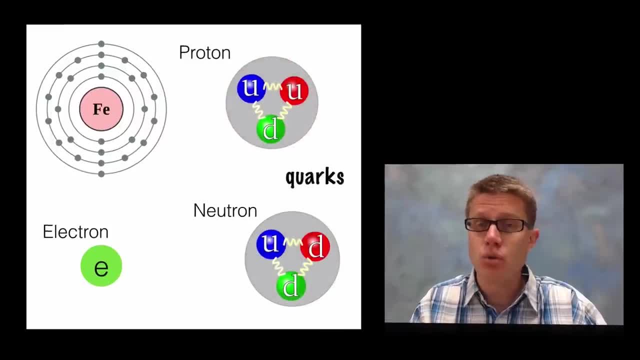 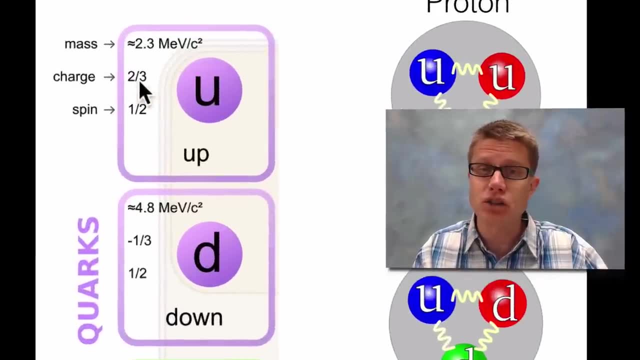 the proton and the neutron to find the fundamental particles, those quarks on the inside. And so here is a data set on an up quark and a down quark. You can see what their mass is, What their charge is And then what their spin is. And so if I want to figure out what 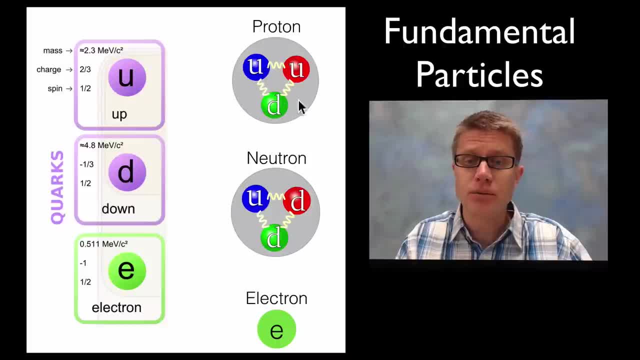 is the charge of a proton. I am going to have to add up all three of these fundamental particles, And so if I take the charge of two up quarks, two thirds times two, that is four thirds, And then I am going to subtract the charge of one down quark, which is going to be four. 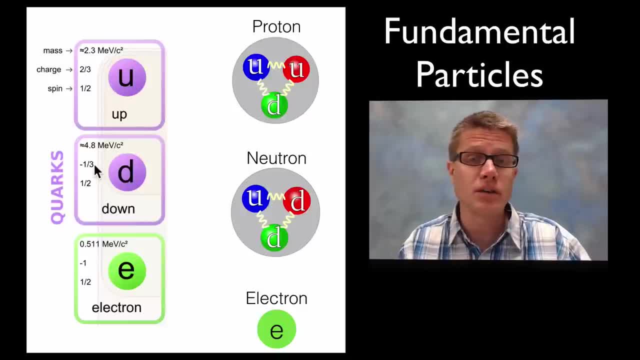 thirds minus a third, I get three thirds or a positive one charge of a proton. It is coming from those fundamental particles. Likewise, with a neutron, we have got one up which is two thirds positive charge minus two, one third charges for the two down quarks, And so a neutron is going to have no charge. 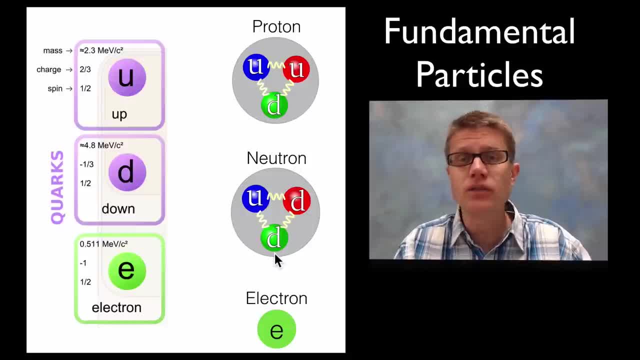 And so, if you are trying to ask a question about the behavior of protons and neutrons at this really, really tiny level, we have to understand what they are made up of. We have to understand these fundamental particles, And so physicists have come up with this standard. 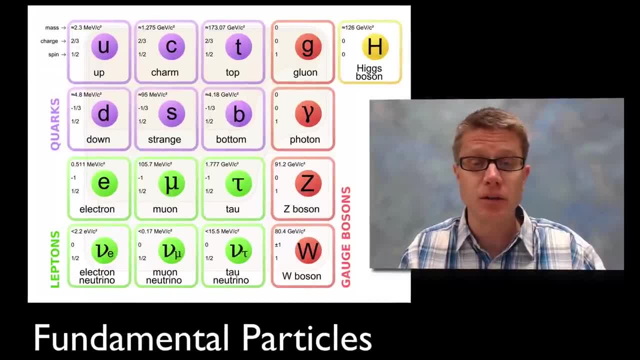 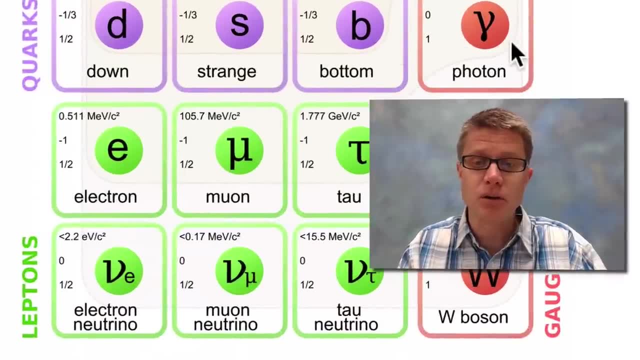 model of understanding matter at the subatomic level, And it spawned all these fundamental particles, Some you are totally familiar with, And so we have got an electron, for example, or a photon, Some you have just a little bit about, like these six types of 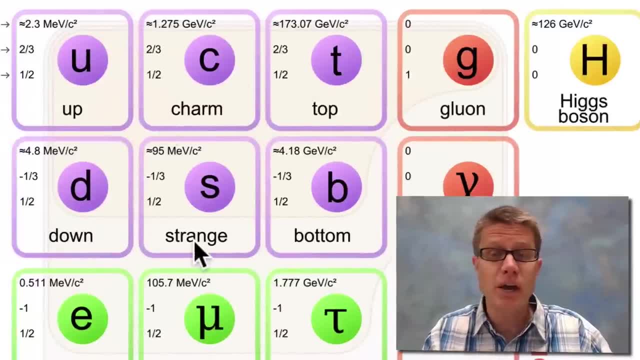 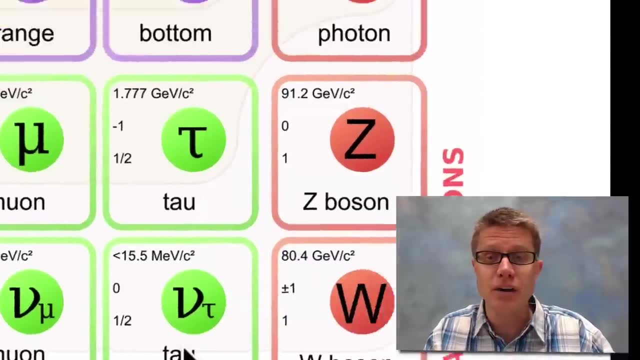 quarks that make up matter, But some are brand new to you and are brand new to science. For example, the top quark was discovered in 1995.. The tau neutrino in 2000.. And, if you have been reading the paper, the Higgs Boson was discovered in 2013 using the Large Hadron. Collider, And so you do not have to memorize all the top quarks. It is all about the subatomic particles. If you don't have any questions about the supertron in this book, you are welcome to do so. So that is where a monopoly of these fundamental particles can be found. 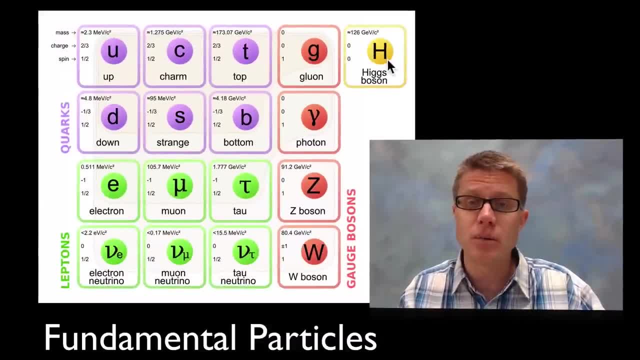 And so we have got an electron, for example. Or a photon And so we have got a electron, for example. memorize all the charges and masses or the names of these fundamental particles, But you should understand this: The difference between a fundamental particle such as a. 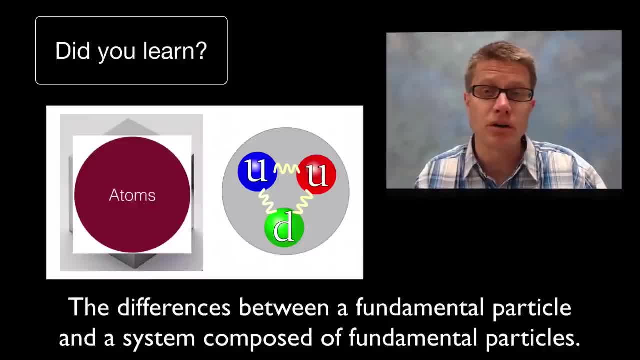 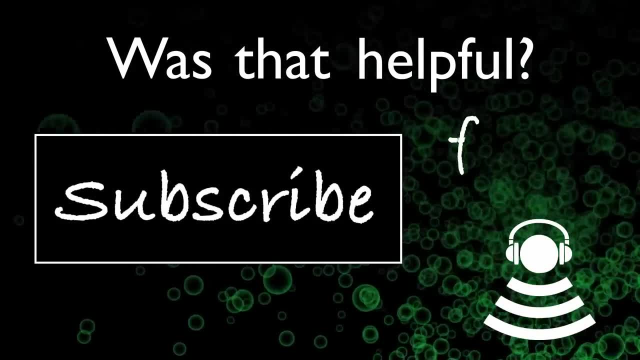 quark and a system composed of fundamental particles, like an atom itself, And I hope that was helpful.